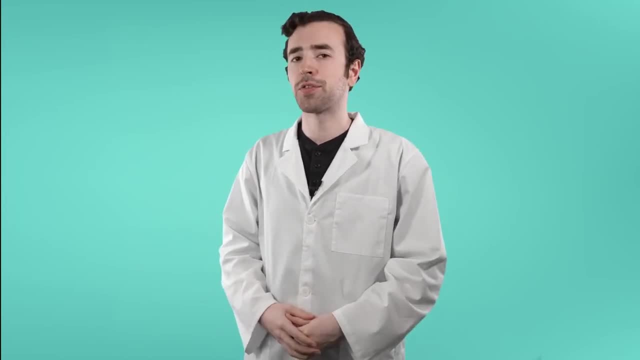 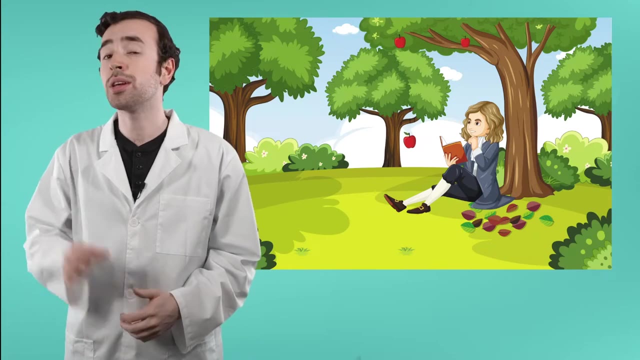 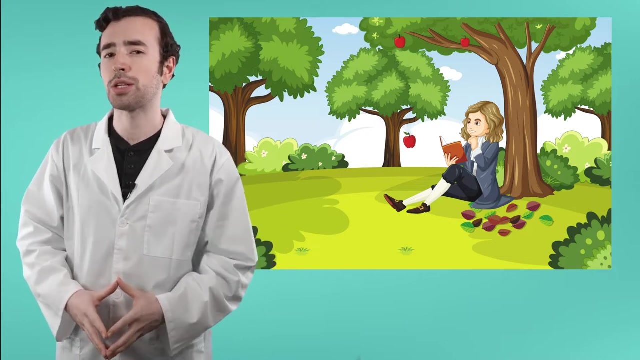 current understanding of gravity once again comes from our good friend CERN. As the story goes, one day Newton was relaxing in his garden when he noticed an apple falling from a nearby tree. Like a good scientist, he came up with a question: Why is it that? 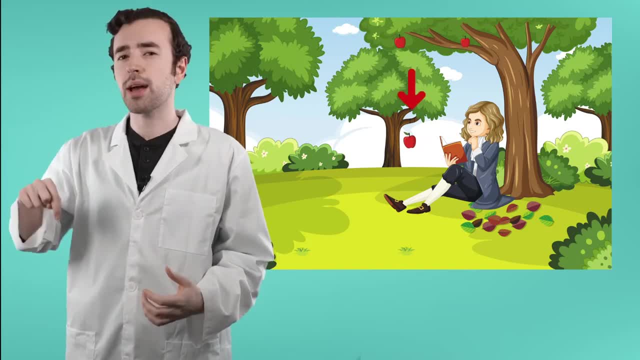 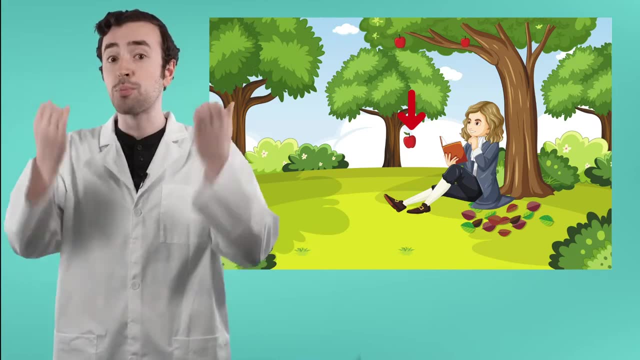 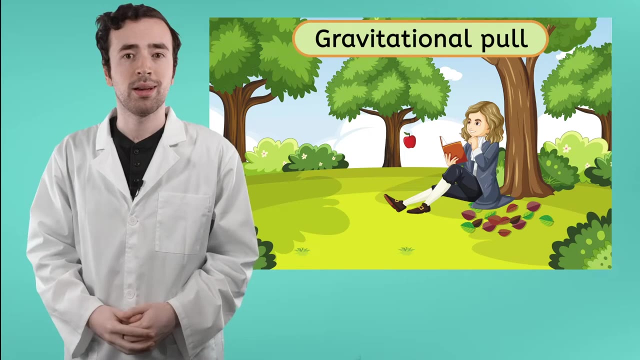 when objects like apples fall, they always go down instead of up or to the side. He knew that there had to be some sort of force that was pulling the apple downward, and he named that force gravitation. Now, Newton was clearly brilliant, but he obviously wasn't the first person to notice. 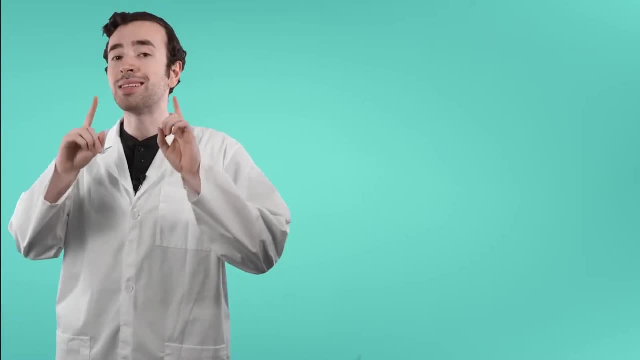 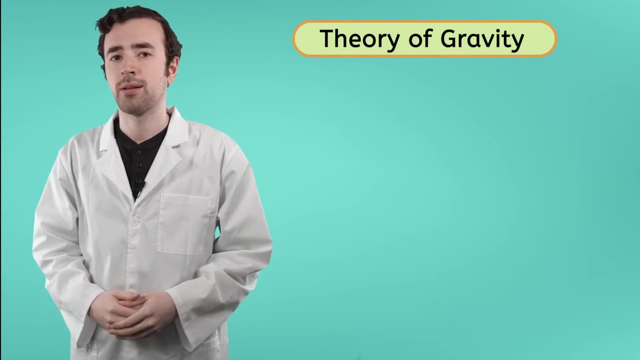 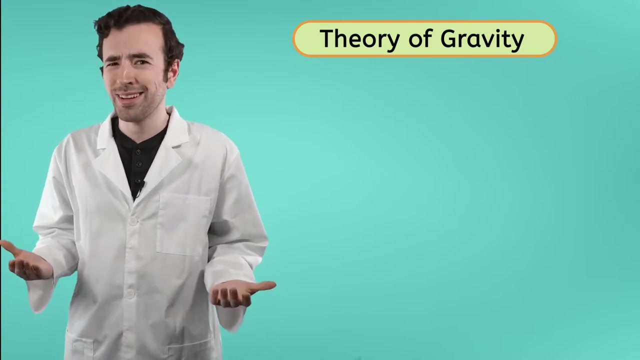 that stuff falls down when you drop it. But what Newton did do was come up with an explanation for what he saw: his theory of gravity. Now I know what you might be thinking, Justin: gravity's just a theory. Well, yeah, but it's. 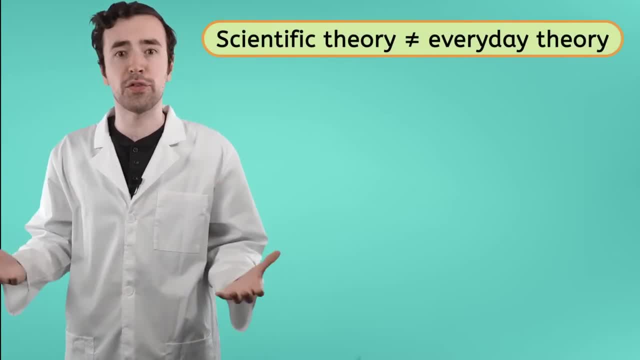 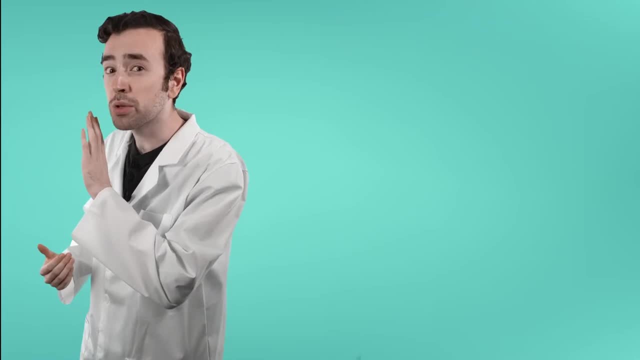 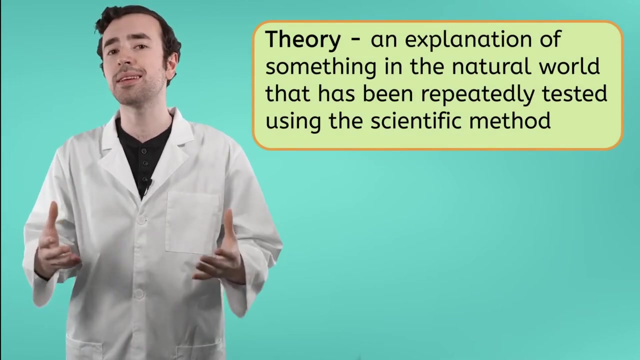 a scientific theory. It's not an everyday life theory like, say, my theory for who left the milk out last night? I think it was a milk ghost. No, a theory in science is an explanation for something that happens in the natural world that we have repeatedly. 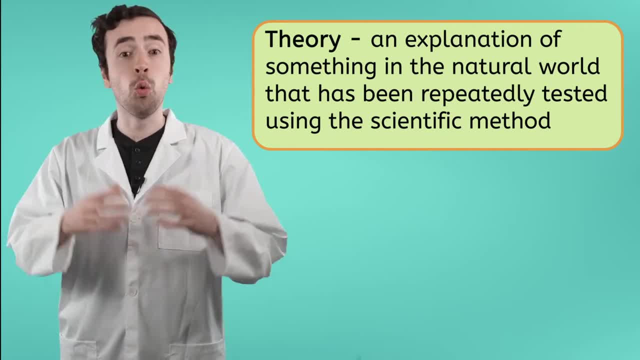 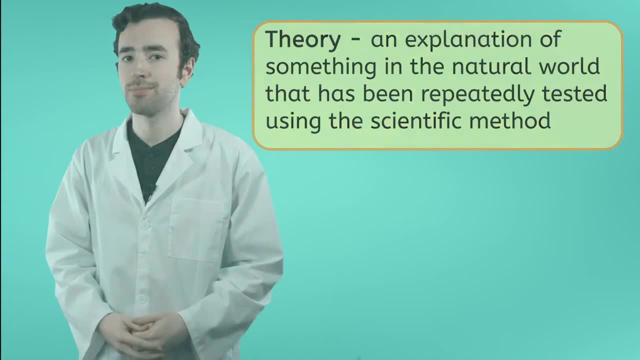 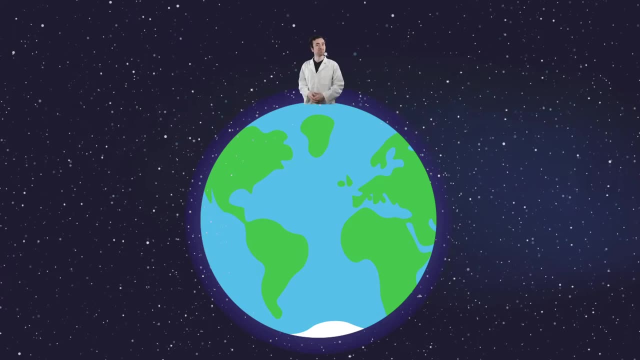 tested using the scientific method. It is overwhelmingly supported with evidence, and so we accept it as truth. Hence the theory of gravity. Without gravity, there would be no life on Earth. It doesn't just pull me back down to my trampoline, It keeps the plants, animals, water, even the air in the atmosphere from 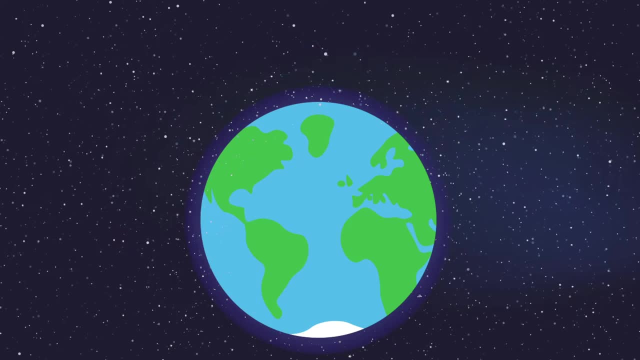 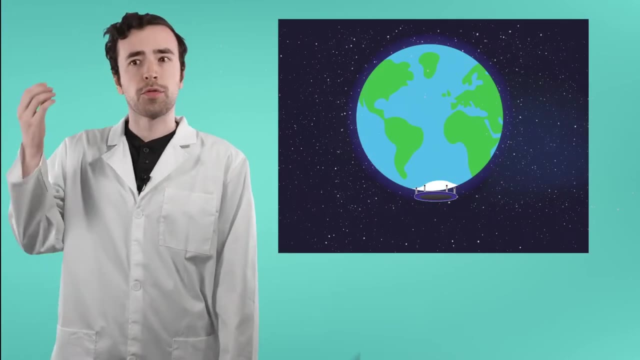 just flying up into space. But does gravity really pull things down? Let's go back to that jumping off the bottom of the globe question. Instead of paying all those exorbitant shipping fees that I would need to travel, I'm going to go back to the 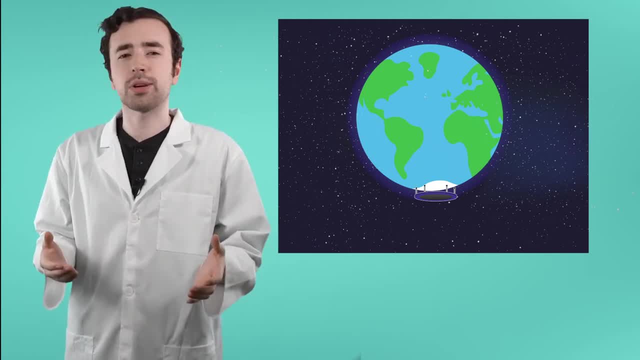 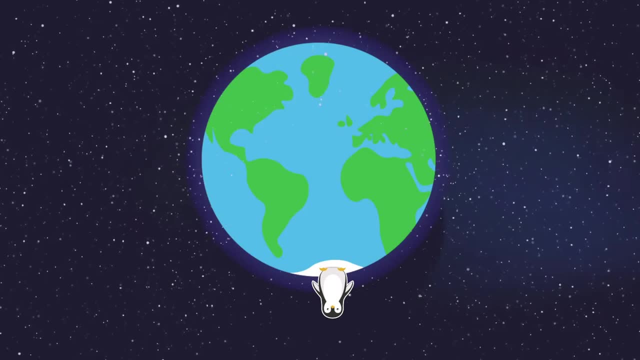 to mail my trampoline to Antarctica. why don't we just look at something that's already there: Penguins. Penguins can be found in Antarctica, on the bottom of the globe, So if gravity pulls down, why don't they go flying off into outer space? 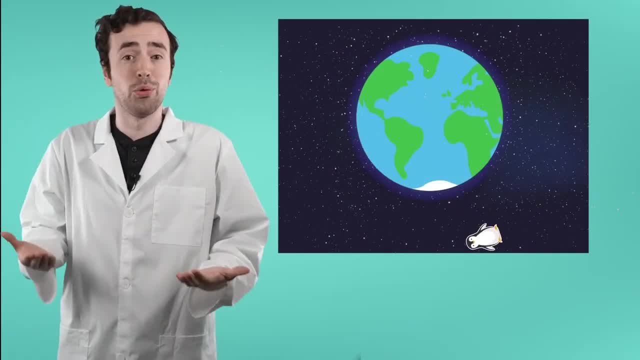 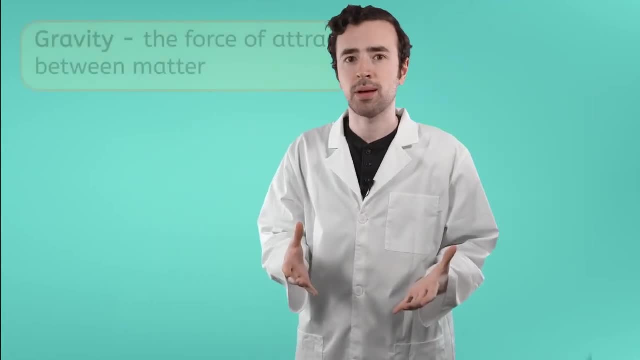 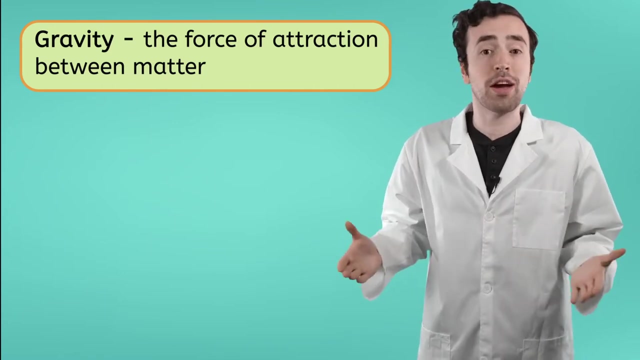 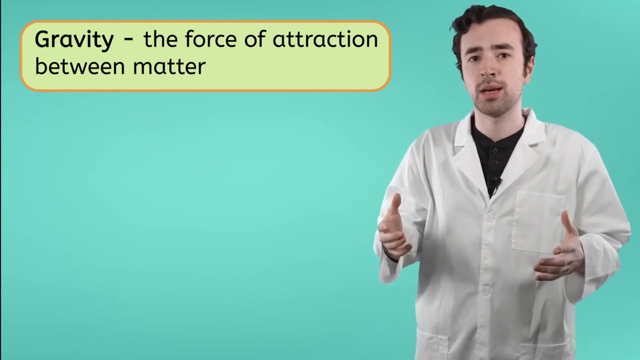 The answer is that gravity doesn't pull things down. It instead pulls things together, Kind of like magnetism. Gravity is the force of attraction between matter. So, yes, gravity is the thing that keeps us down on Earth, but it's not pulling us down- luckily for the penguins. No, the Earth's gravity is pulling you and the Earth together. It's kind of like a toddler: It just doesn't want to let go of his teddy bear. Aw, And this force of attraction doesn't just exist between us and the Earth. 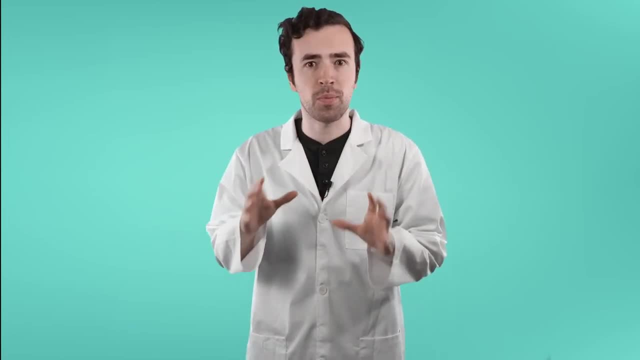 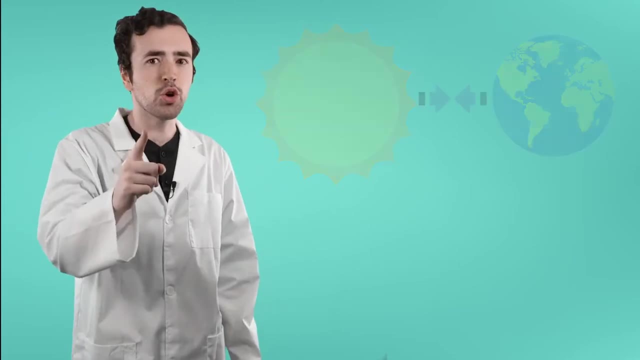 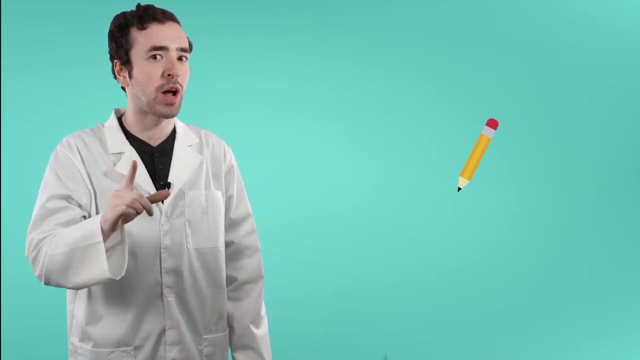 There is gravity between everything with mass. There's gravity between a meerkat and the Earth, between the Earth and the sun, between you and this pencil. You are probably not feeling any force of attraction between you and this pencil, And that's totally normal. 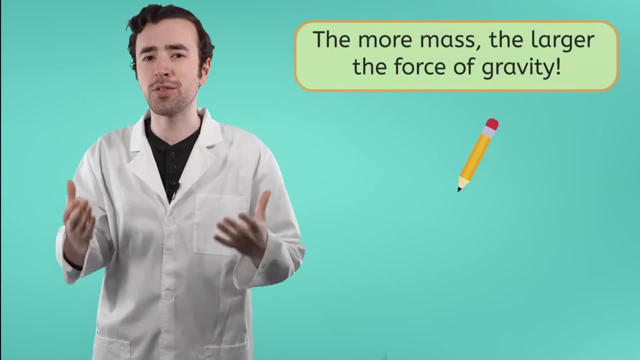 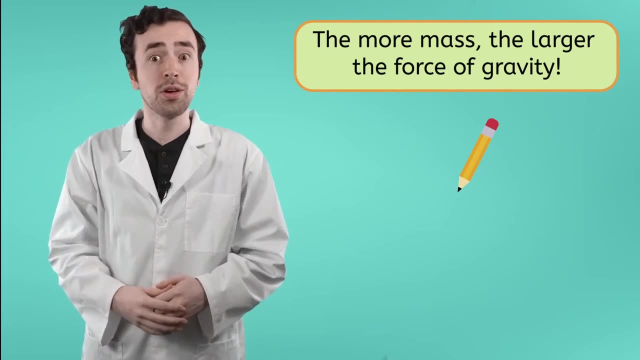 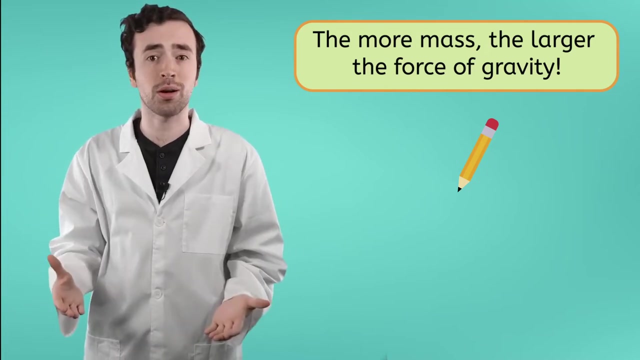 It'd be a little weird if you did, Because the strength of gravity is dependent on mass. The more mass, the stronger the gravity. Earth is really massive, So of course its pull from gravity is gonna be super strong. Neither you or this pencil have enough mass. 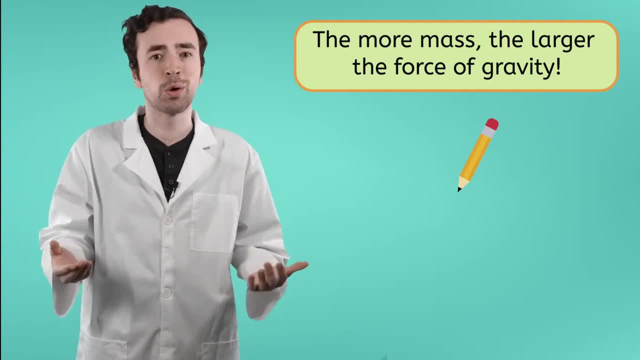 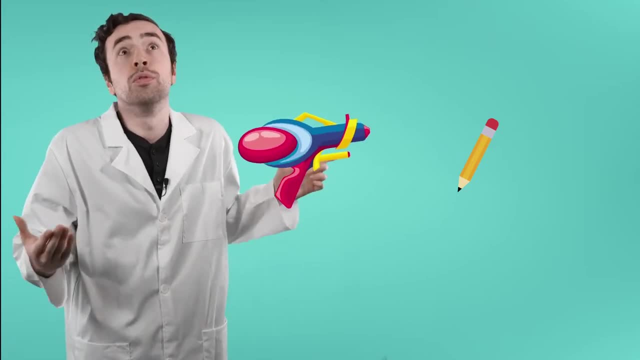 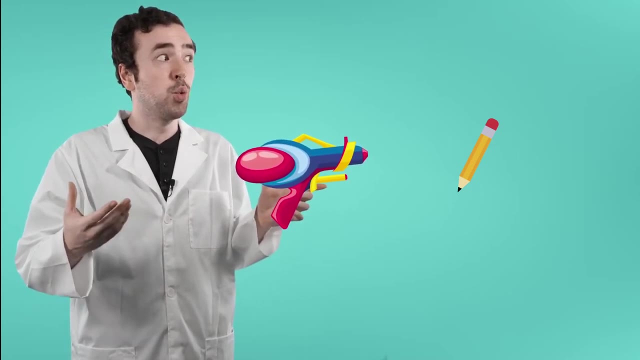 to make the pull of gravity between you two noticeable at all. But if someone were to take, say, a super villain growth ray and grow this pencil so that it was the size of the Earth, then you would feel as attracted to it as you do to the Earth itself. 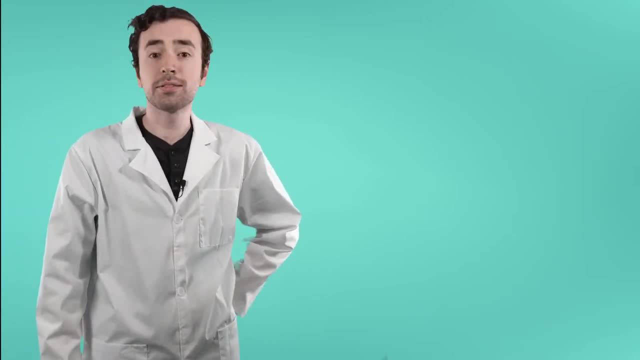 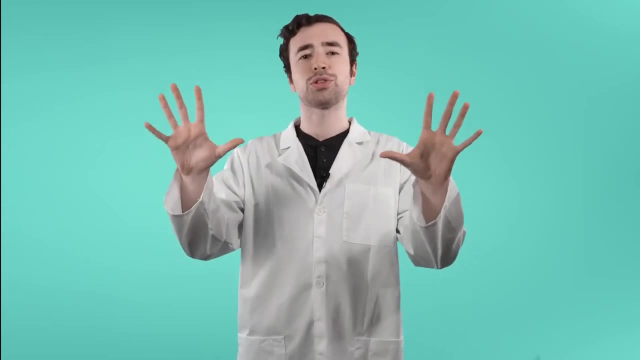 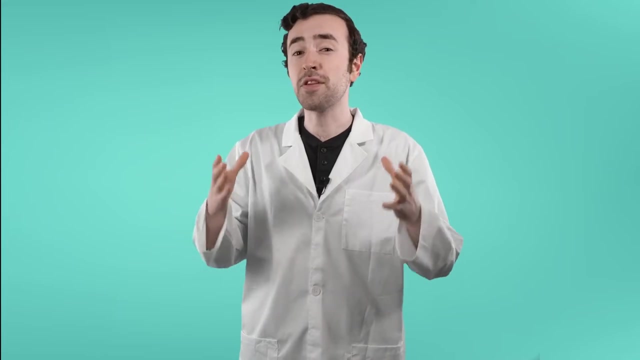 I mean that's neat, right. And as we've seen, gravity isn't just something that exists on Earth. It extends outward, It bends out into the solar system and to the universe beyond. Can you think of something that's even more massive than the Earth? 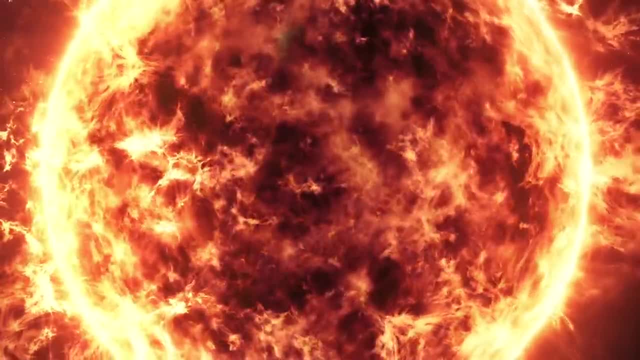 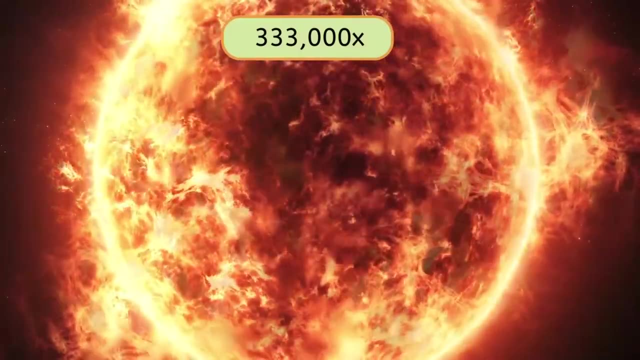 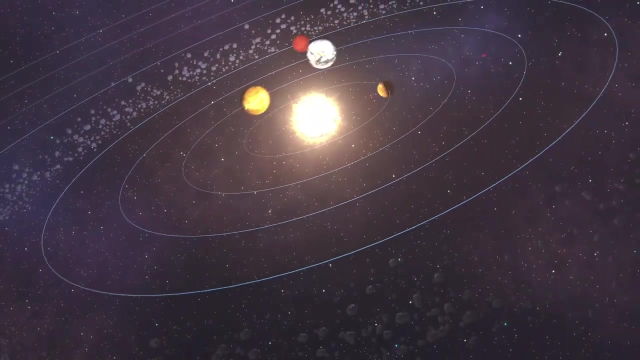 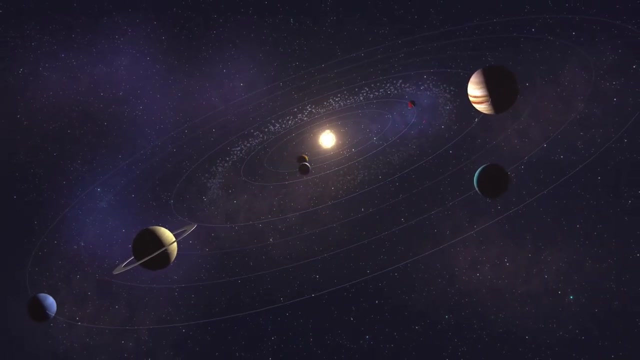 Well, the Sun for one. The Sun is 333,000 times more massive than the Earth, so its gravity is also way stronger. The Sun's force of gravity is so strong. it's actually what keeps all the planets in our solar system in orbit around it. 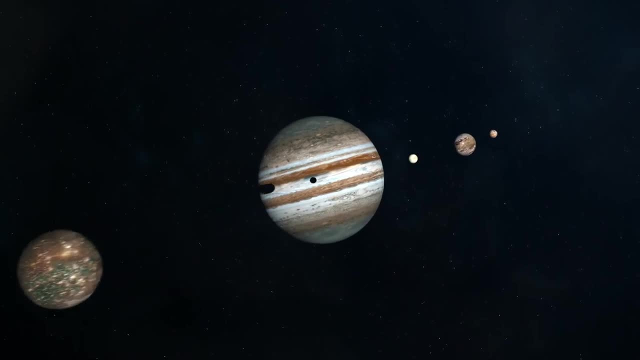 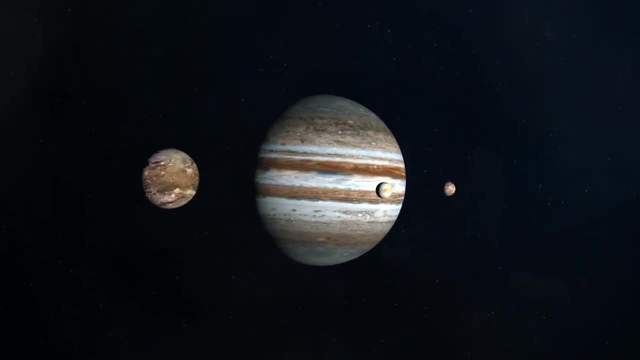 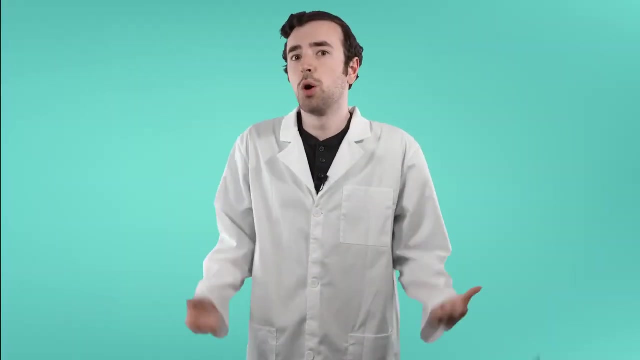 While not nearly as big as the Sun, Jupiter is also much more massive than Earth, giving it a much stronger gravitational pull. That's why it has more than 80 moons orbiting its mass compared to Earth's one. Since most of us live our whole lives down here on Earth, we're not going to be able. 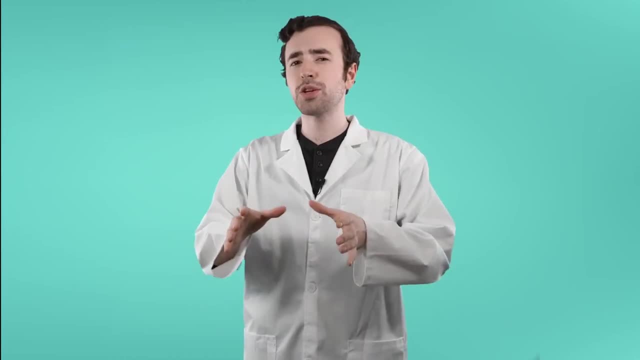 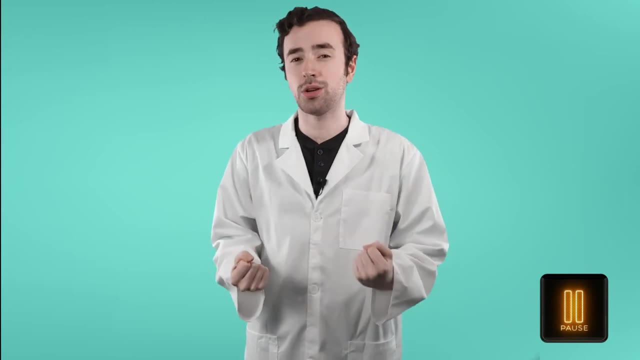 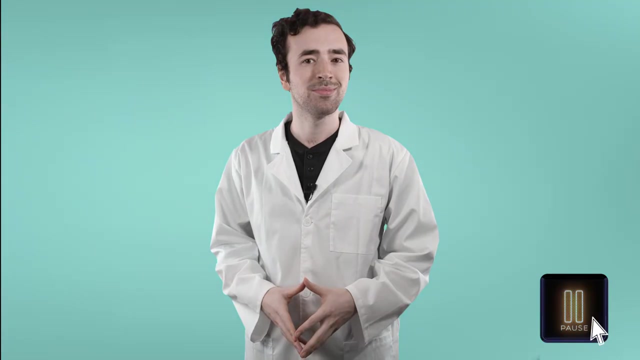 to get used to its gravity. What do you imagine it would feel like to go live somewhere like Jupiter, where the force of gravity was so much stronger? Pause the video here to write down your thoughts in your guided notes. So the force of gravity is dependent on mass. 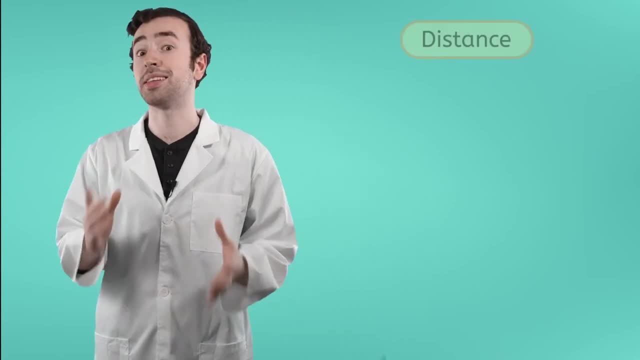 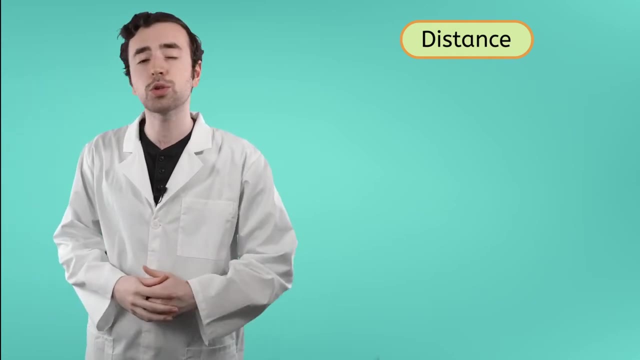 But it's also dependent on one more thing: Distance. The farther away it is from Earth, the farther away it is from Earth. Distance, Distance: The farther away it is from Earth, the farther away it is from Earth. But the more two objects are, the weaker the force of gravity will be between them. 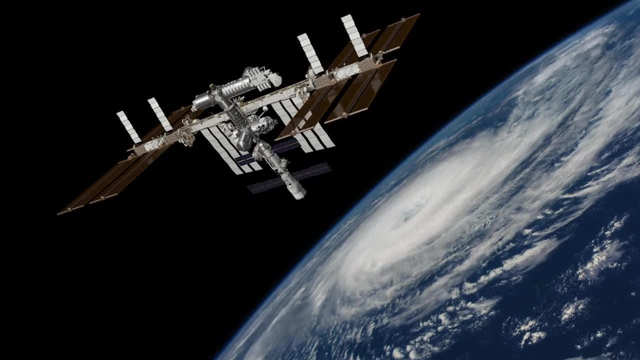 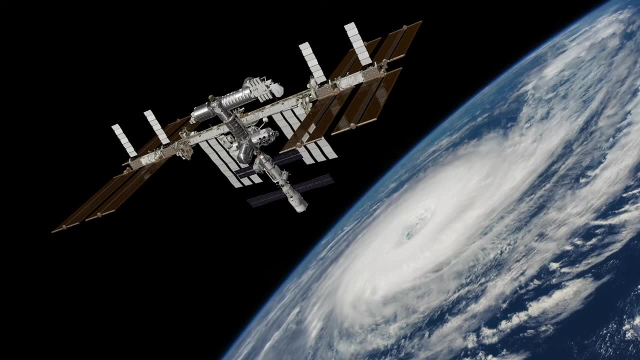 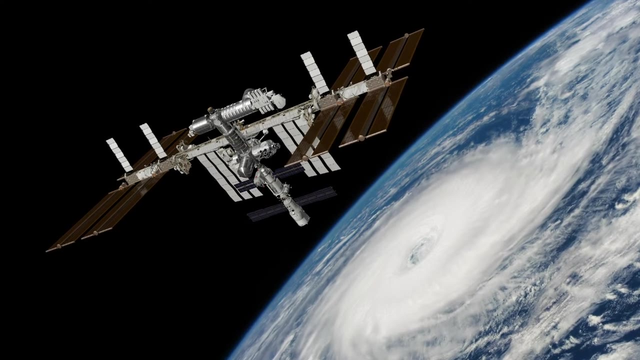 This is demonstrated by what astronauts experience when they leave the Earth's surface. For example, astronauts aboard the International Space Station are still in Earth's orbit, so they're still experiencing Earth's gravity, But because they're about 260 miles away from the surface of Earth, the force of gravity 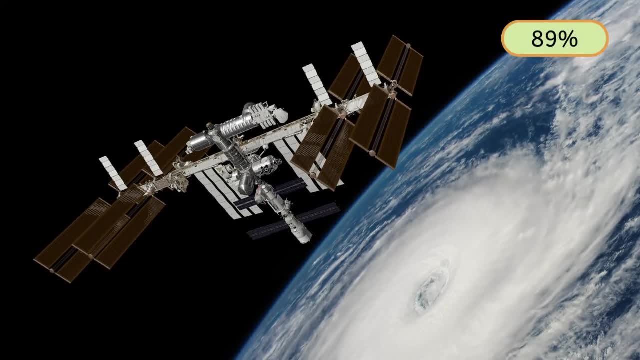 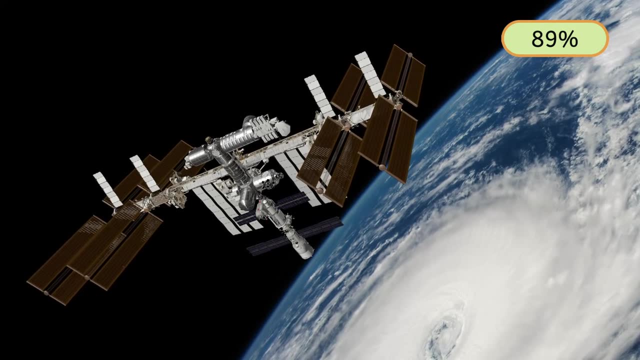 is only about 200 kilometers, about 89% as strong as what we experience on the ground. If they continued past the space station, the gravitational pull between the astronauts and the Earth would continue to get smaller and smaller until they didn't feel it at. 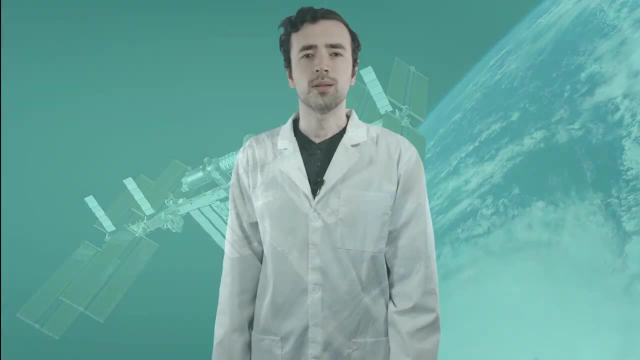 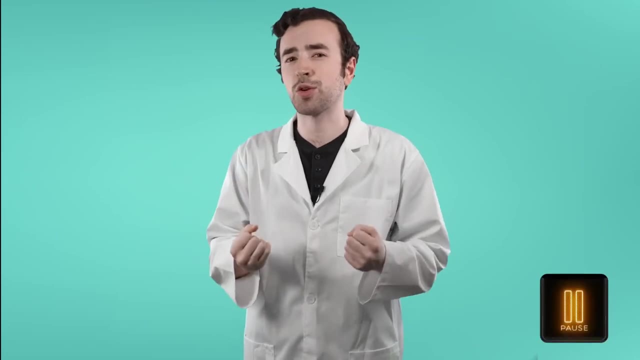 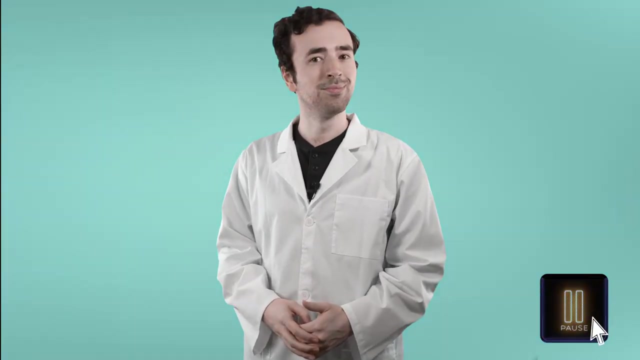 all, What do you think it would feel like to move so far away from Earth that you don't even feel its gravitational pull anymore? Pause the video here to jot down your ideas in your guided notes. Let's review everything we've learned today. 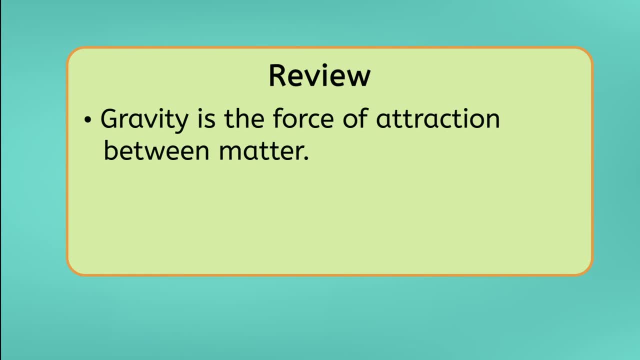 Gravity is the force of attraction between matter. The strength of a gravitational pull is determined by mass and distance. The more mass an object has, the stronger the force of gravity it has. The farther away an object is, the weaker the force of gravity.